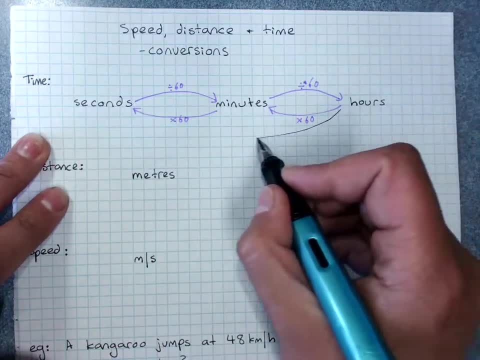 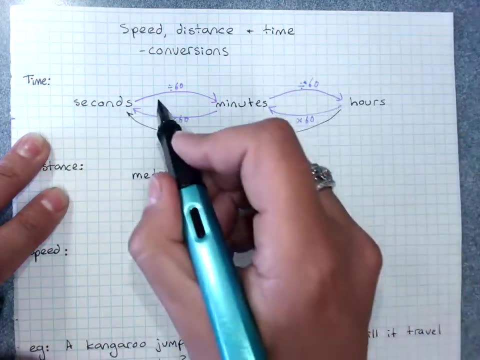 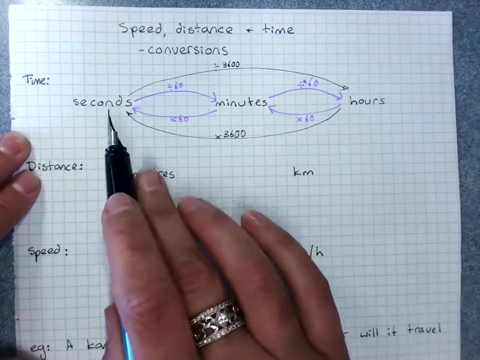 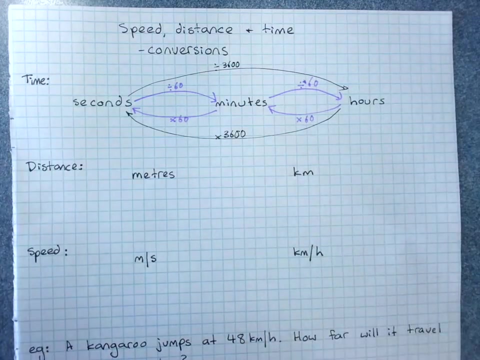 And times by 60 again, And that all works out to times by 3,600. And it's the opposite. to go back the other way: Divide by 3,600. So you can convert seconds into minutes, or seconds into hours, or minutes into hours. all the way, Any combination you need. 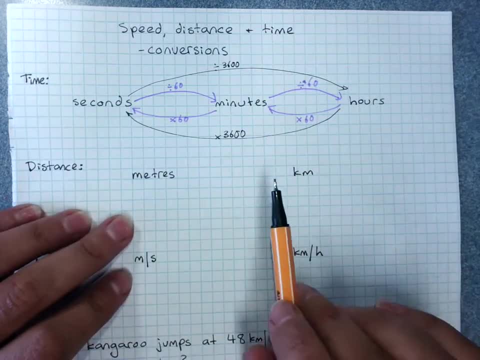 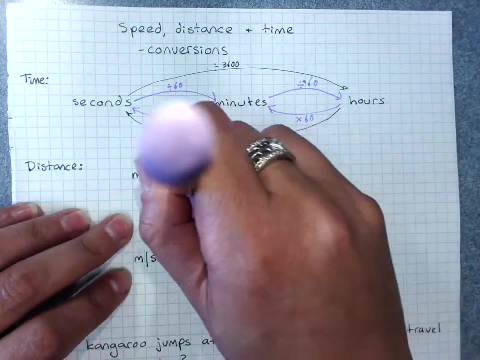 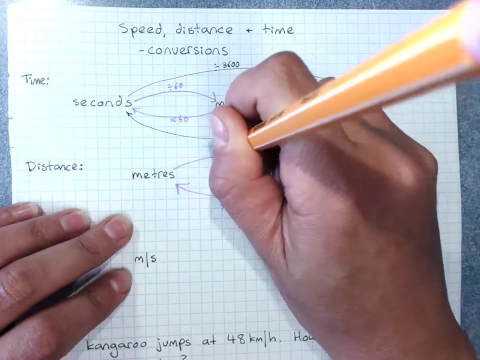 Distance is much easier: Meters and kilometers. There's a thousand, There's a thousand meters in a kilometer. So you can see, if I had one kilometer to go to meters, I'd times by a thousand, And that means to go from meters to kilometers. I would do the opposite, I'd divide by a thousand. 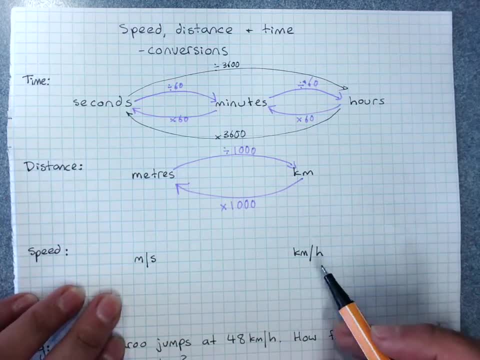 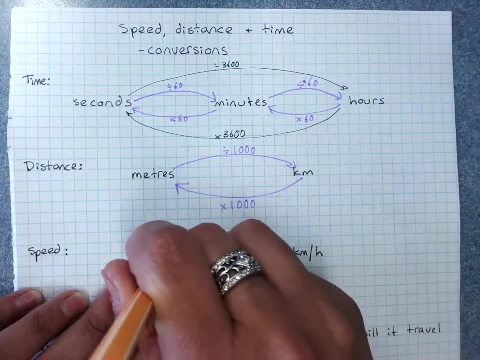 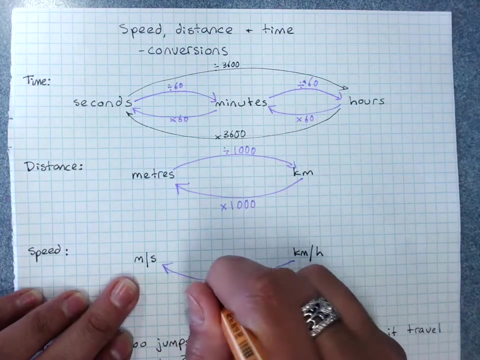 Now meters per second and kilometers per hour converting speed. you can convert it all separately, but there is a shortcut: Kilometers per hour back to meters per hour. Kilometers per second Divide by oh, I should have put them in the same order, I'm sorry. 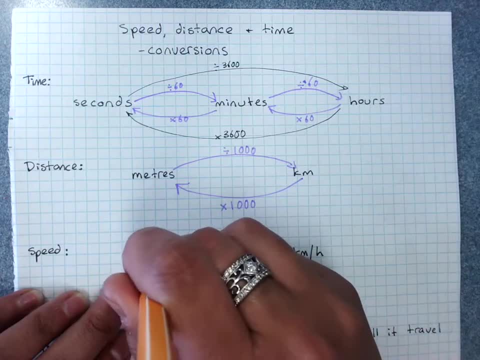 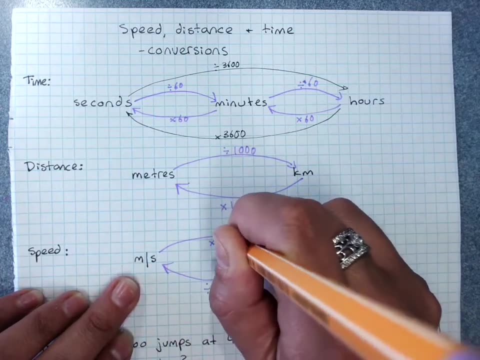 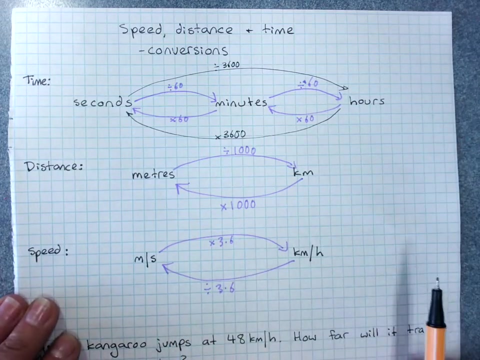 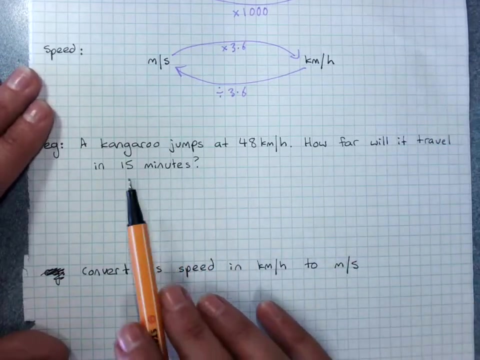 Divide by 3.6.. Meters per second to kilometers per hour. Do the opposite Times by 3.6.. So if you need to convert speeds, we can use that one. So some example situations where we might need this. 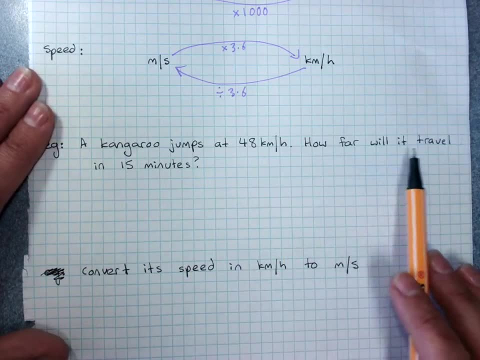 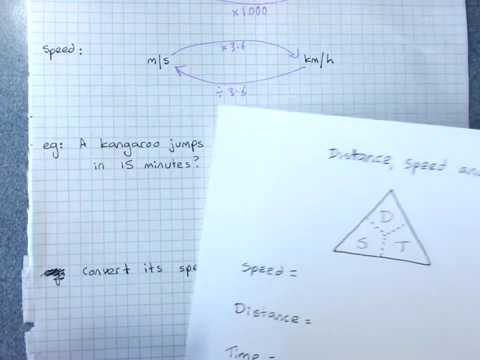 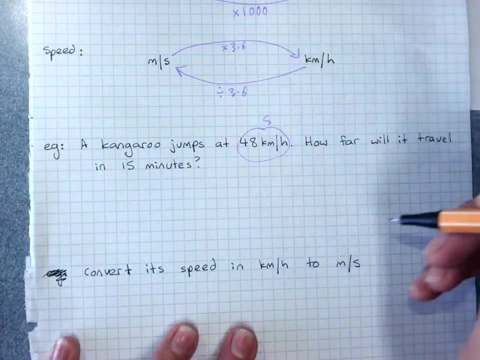 A kangaroo jumps at 48 kilometers per hour, How far will it travel in 15 minutes? So, of course, first up, we use our speed-distance-time triangle. We want to know we've got its speed, we've got its time, how far we want the distance? 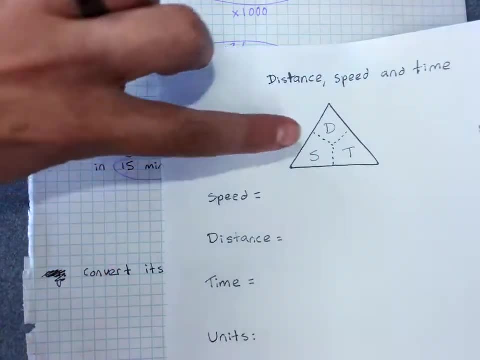 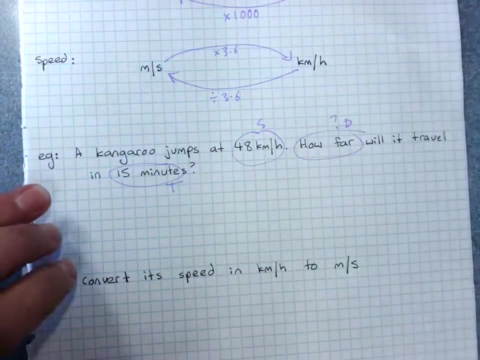 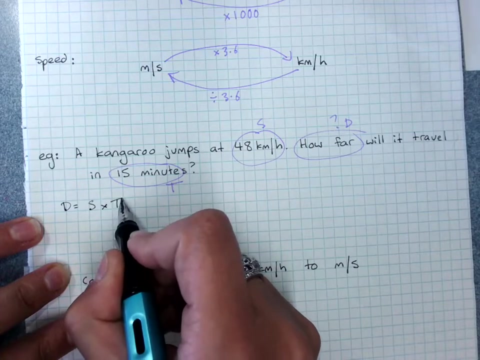 So we get our speed-distance-time triangle, We cover up distance and we discover that speed times time because they're next to each other. So we write our formula of speed. sorry, distance equals speed times time. But we check our speed is in kilometers per hour. 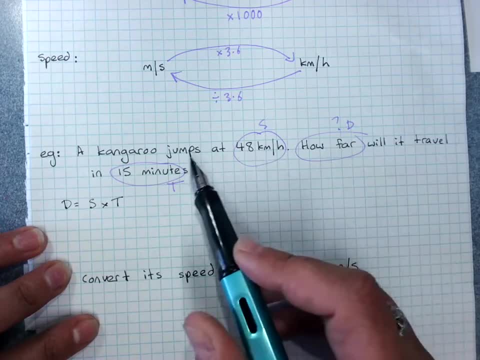 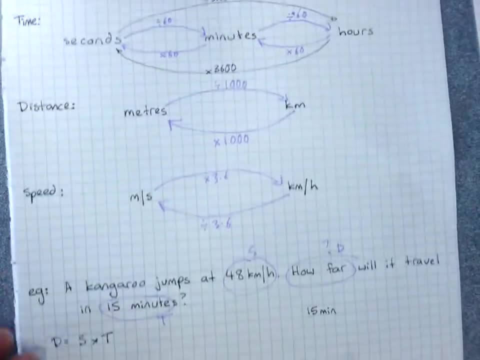 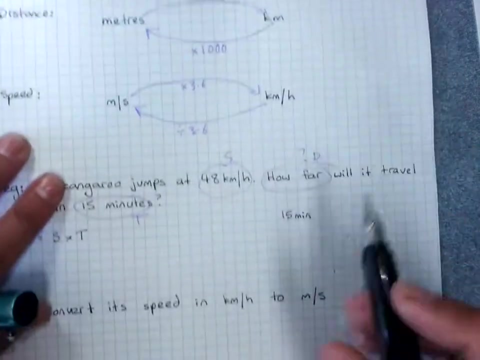 Our distance will work out in kilometers, but our time needs to be in hours. So over here, 15 minutes. We need to work out 15 minutes and change it to hours. So we'll divide by 60 to go from minutes to hours.